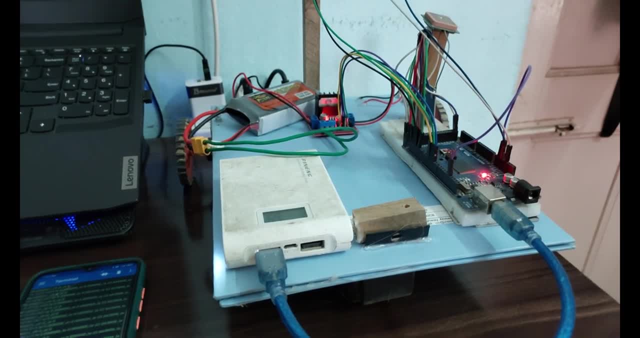 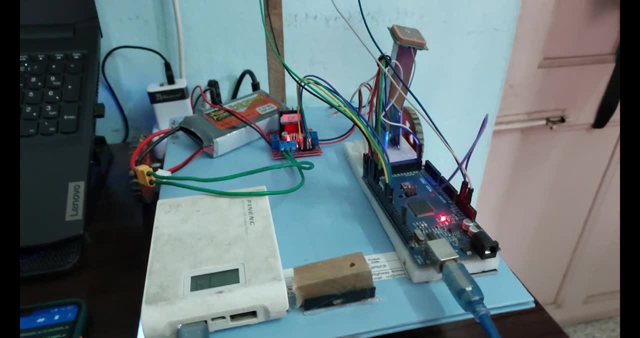 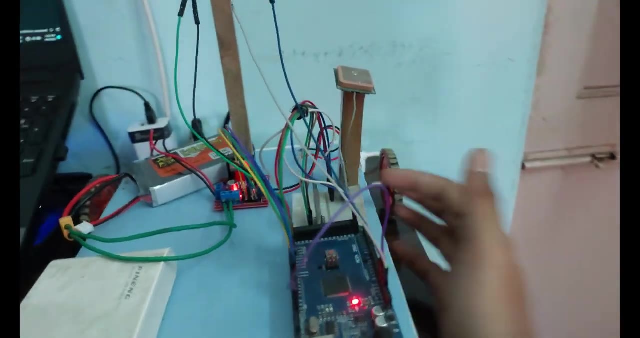 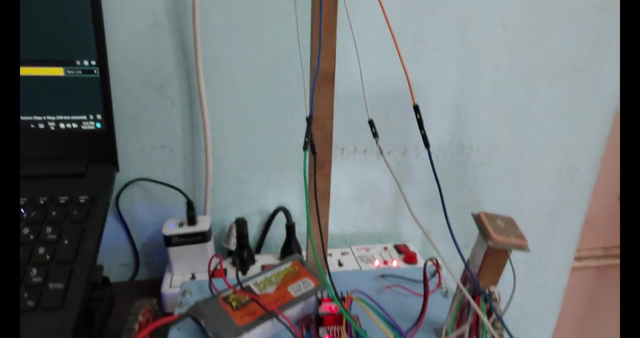 Hello friends, welcome back to another video on this channel. In today's video I will show you how I made this and how you can make yourself an autonomous robot. So the basic principle of an autonomous robot is actually quite simple. So basically, it takes the coordinates, its current coordinates, using this GPS here, And it also has a digital compass up here which it uses to get its current heading, And then you can put the coordinates of a location where you want it to go. You 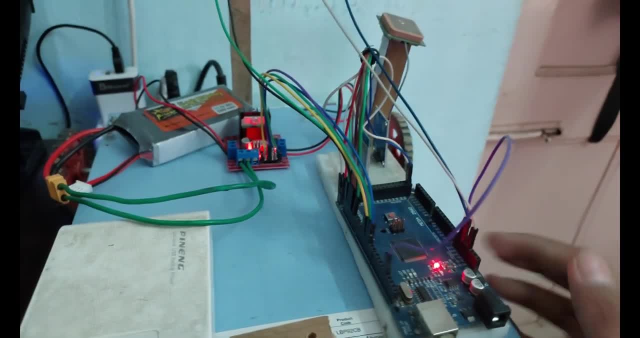 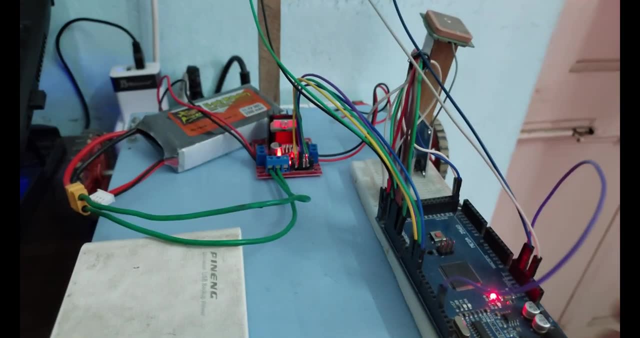 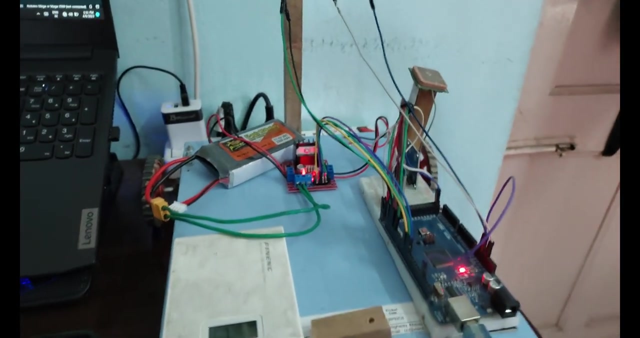 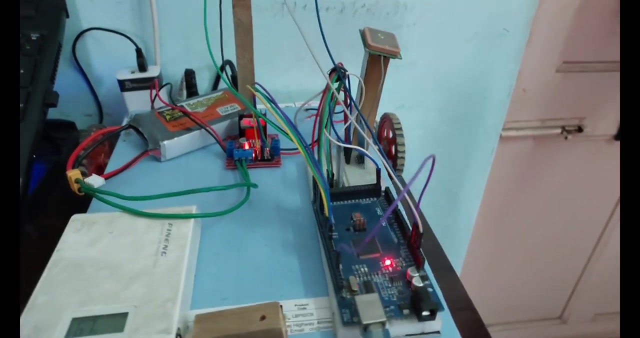 can use the computer and basically the microcontroller here just calculates its current position and where it wants to go, It finds out the error heading and then it uses this motor controller to drive these two motors here and here to move the robot, to make it move to the position where you want it to go according to the GPS coordinates. Additionally, we have a 8605 Bluetooth module here to basically 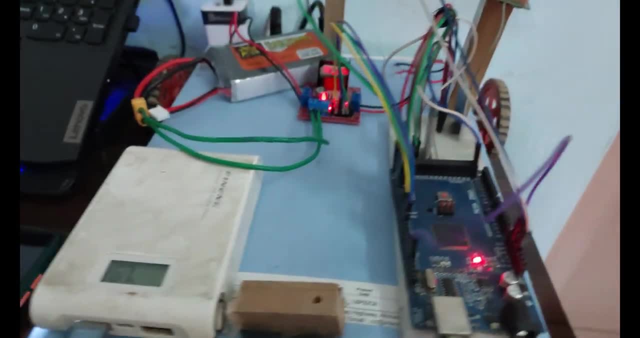 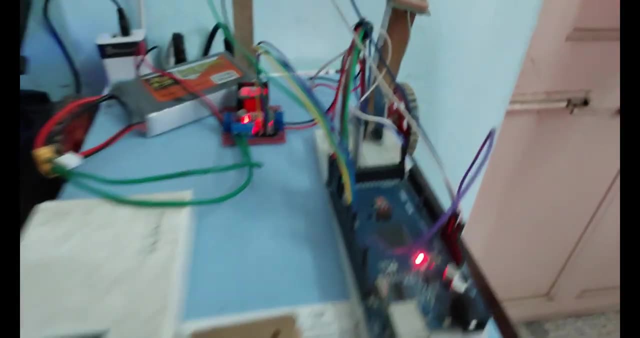 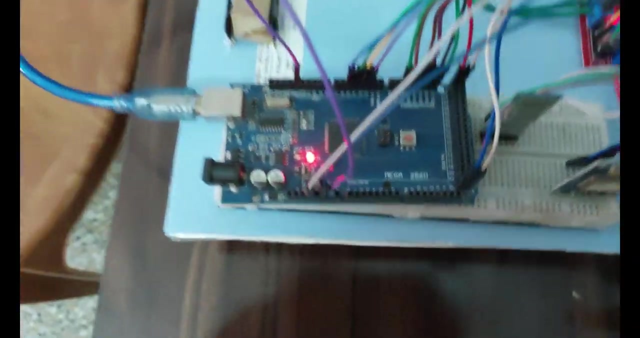 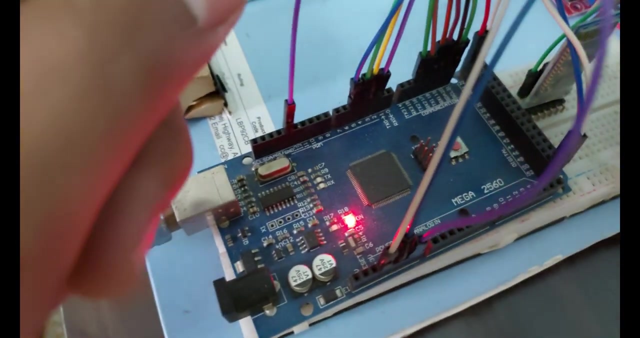 just monitor it using serial, Bluetooth serial. I will leave the link down below for the serial monitor app I'm using on my phone. So let me just show you a little bit about this wiring. So first of all we have the Arduino mega. First thing you will notice is this wire which is connecting to ground on one side and on the other side it is going to digital pin number 13.. This is just your like, just to basically stop the microcontroller from moving as soon as you power it on. So you can 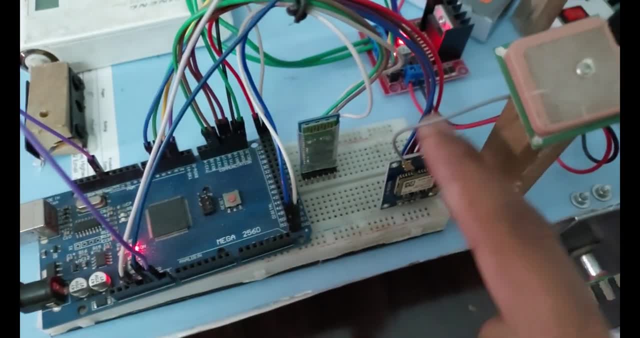 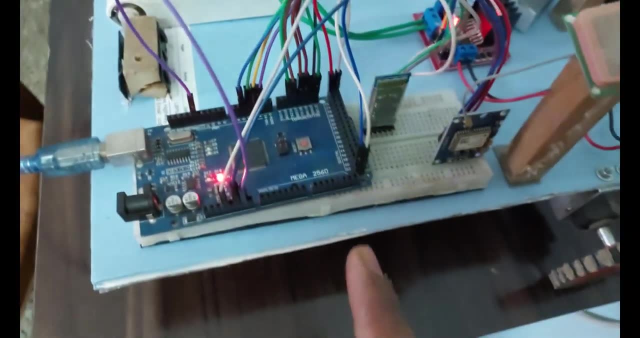 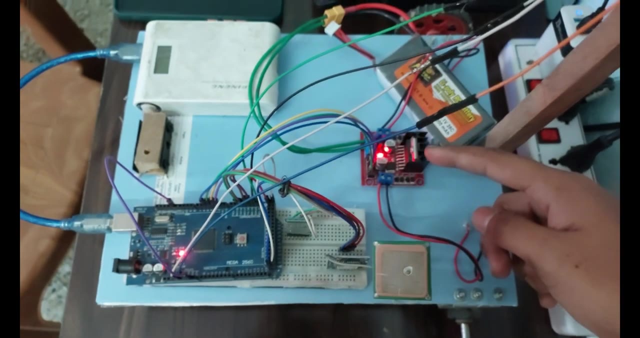 it on so you can get it set up and have the gps here, which is the new 6m v2. this gps get the coordinates and stuff. you can set that all up. once you're done, you basically just disconnect this from ground and the microcontroller will spring into action. it will then power up the uh. this: 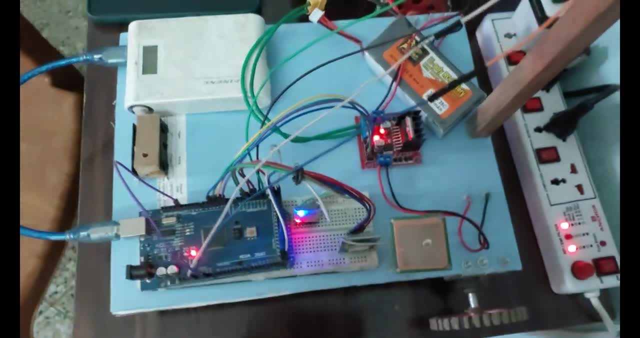 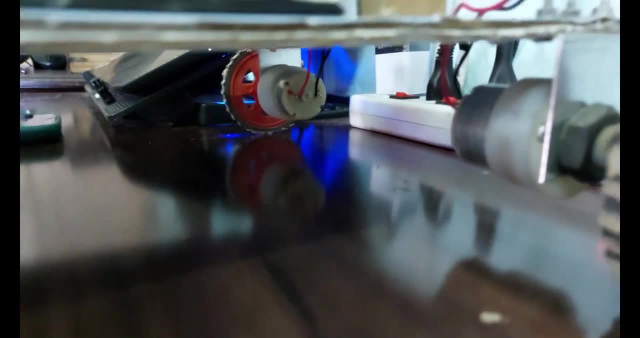 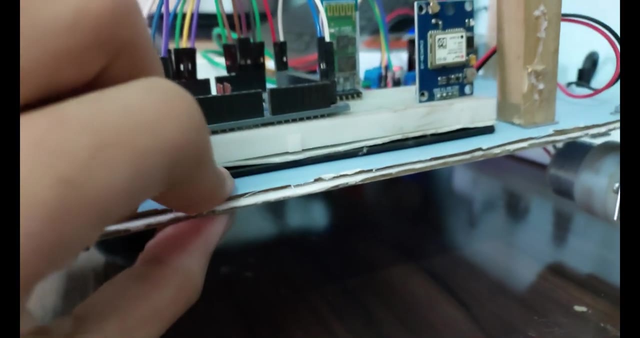 motor controller, which here is the l298n. this motor controller will then power the two motors. i'm using 12 volt geared, 150 rpm motors and i'm just using a set of wheels. there's actually a bit story behind these wheels. i'll tell that in just a bit. this is just some normal, uh, hardwood board. 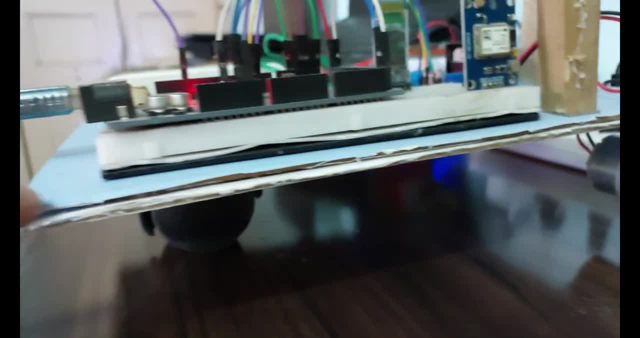 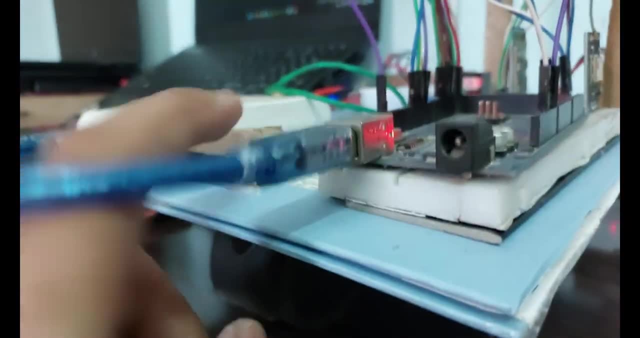 i've just used two slayer dust, two layers stacked up, because otherwise this is quite flimsy. now, down here, the third wheel is just your normal swivel wheel. i've just mounted it using this piece of wood up here. the entire microcontroller, the bluetooth module, as well as the gps. 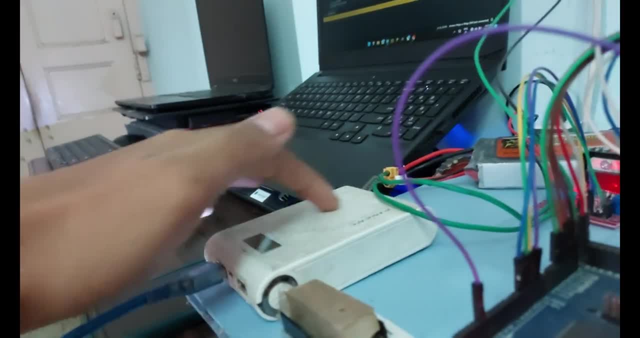 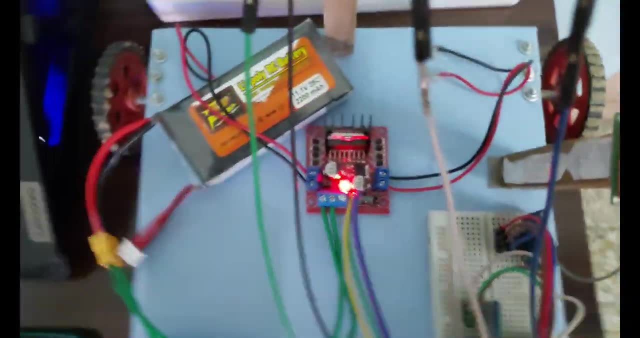 also, the car compass is powered up using this power bank. here it just plugs in via usb onto the microcontroller which powers up everything on the electronics side, and then this motor controller, since it needs 12 volts. how this micro, this power bank, as well as everything else, is 5 volts and the 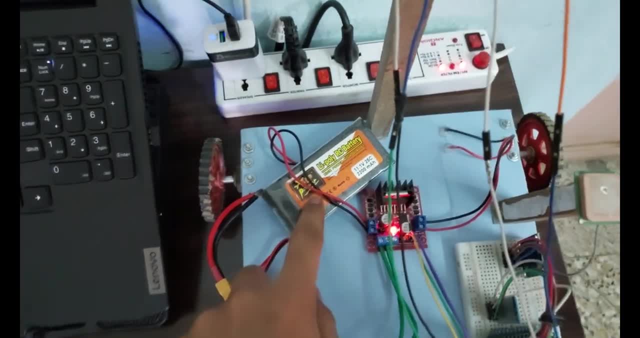 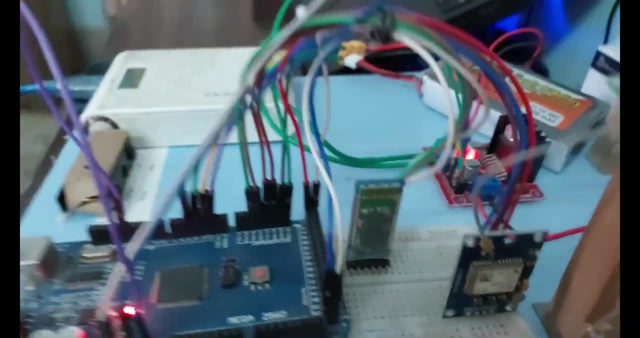 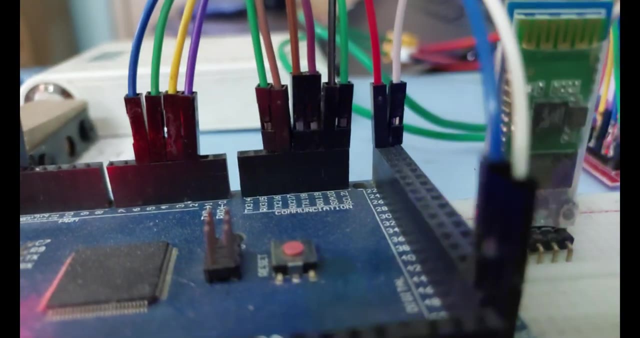 compass is 3.3 volts. we simply are using this 11.1 volt lipo battery for connecting up to the motor controller. now, additionally, for wiring the gps module is wired up into- uh. sorry, the gps is wired to uh serial one. serial zero has to be left open. that is for 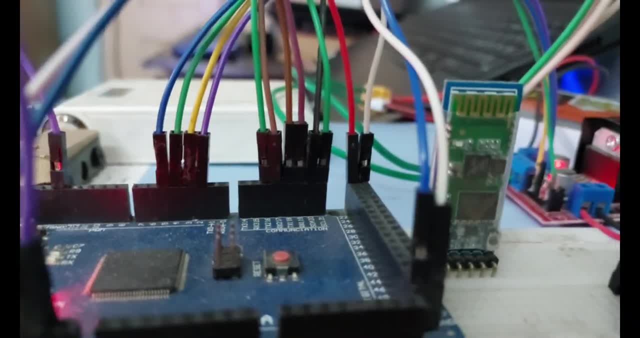 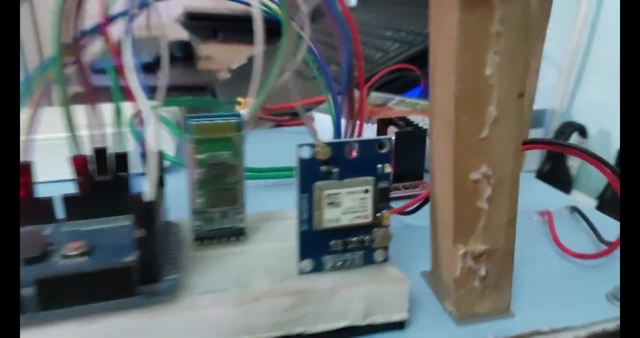 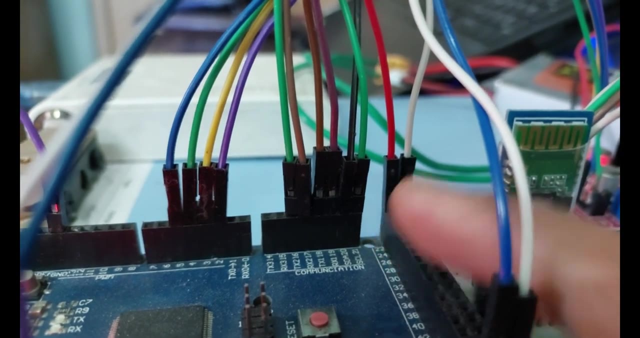 communication with the computer. the gps is con. sorry, the bluetooth is connected to serial one, uh, two, sorry, the so for wiring the gps is connected onto serial one, the rx and tx, as you can see rx1 and tx1 there, pin number 19 and 18.. that is the gps, the serial 2, which 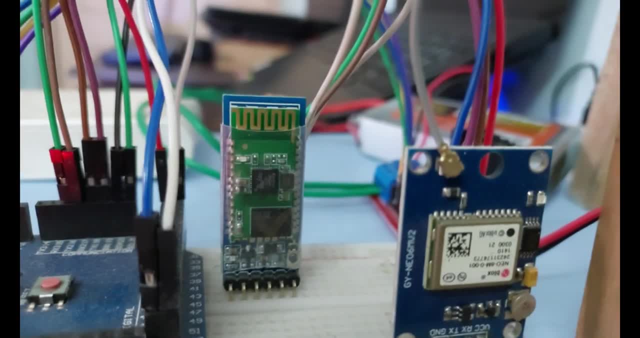 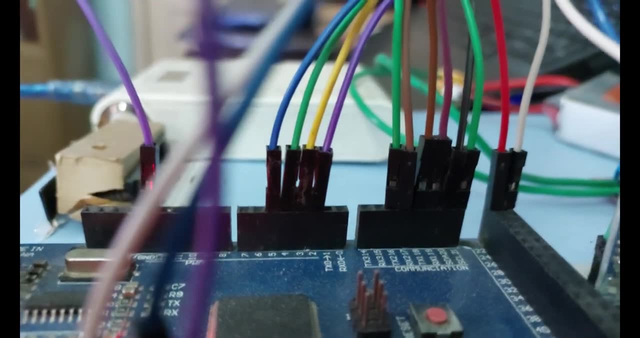 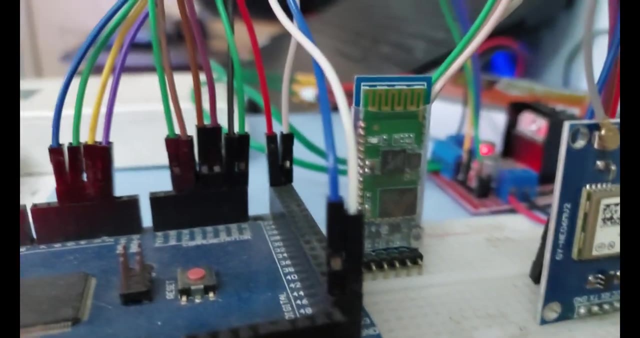 17 and 16 is the bluetooth module, and then you have to leave serial zero- that is our zero- and one pin open, that is for communication with the computer. there is another serial port free, which is serial 3, that we are not using. however, if you want to add something onto this, you can. 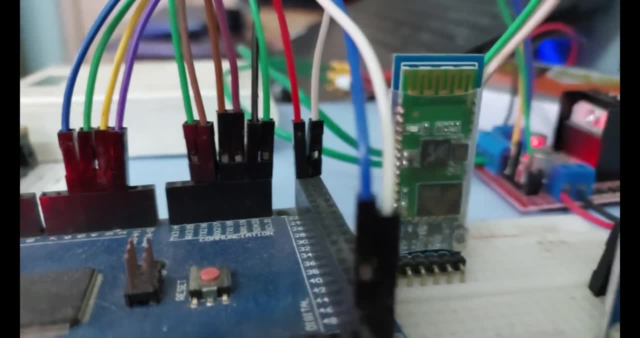 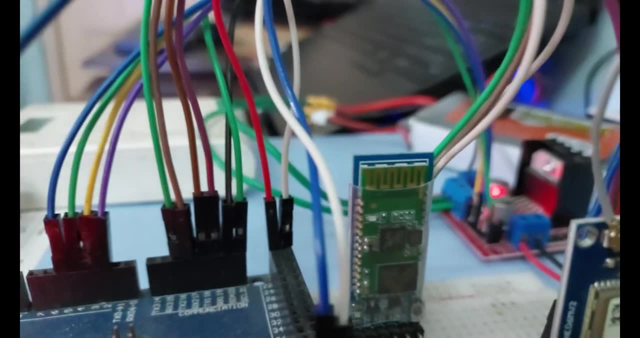 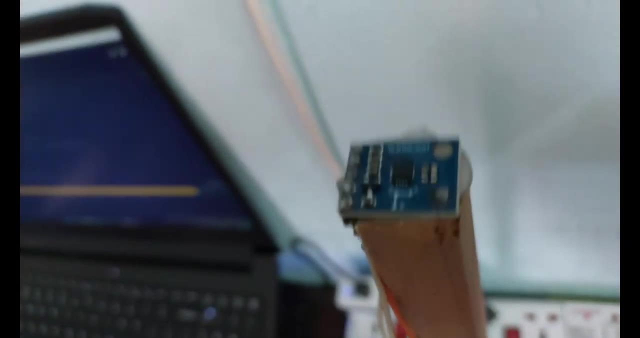 use that for communicating to the compass. we are using i2c, so we are using the sdi and scl. as you can see, this green and green and black wire is connecting up here, passing on through to the compass here. this compass, by the way i think i mentioned, i will mention again this is: 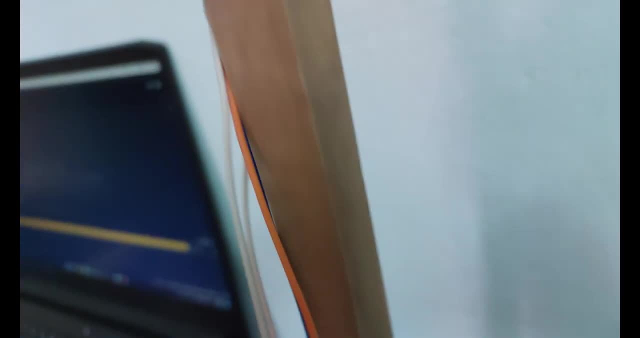 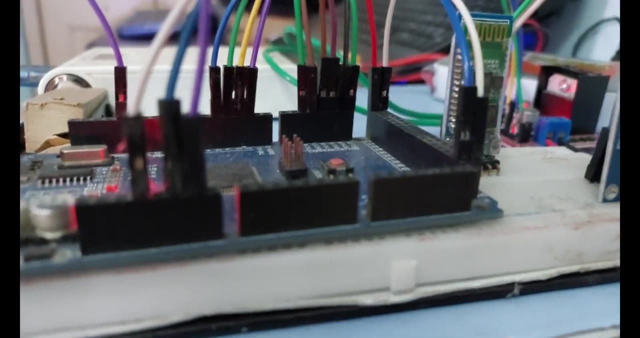 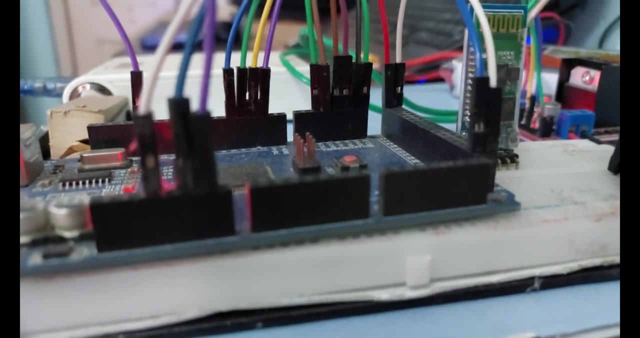 the gy273 hmc5883l. however, a common thing about these hmcs is that they are actually qmcs, so they will not be recognized by the hmc library. this was the case with mine, so my code is running qmc library but, however, i will leave the hmc code as well. 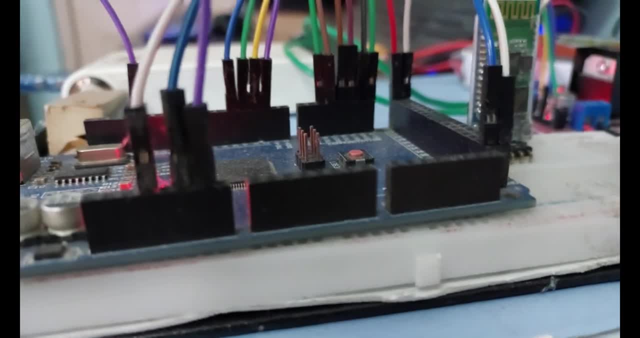 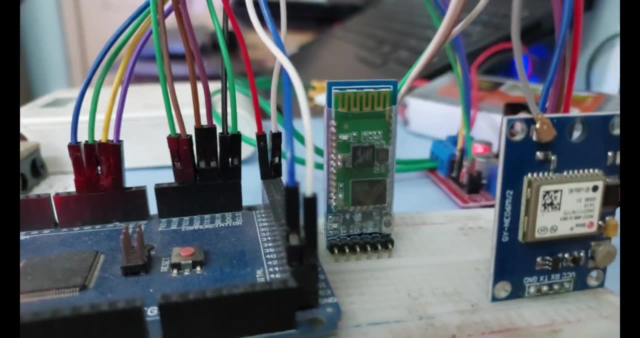 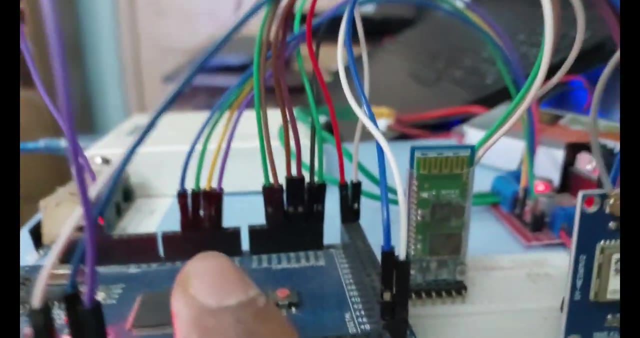 along with the qmc code. so if you get the hmc so you run the other code. other than that, one more thing to notice, a note about the gps and the bluetooth module wiring is that you have to plug the rx of the device module to the tx of the microcontroller and the rx of the microcontroller. 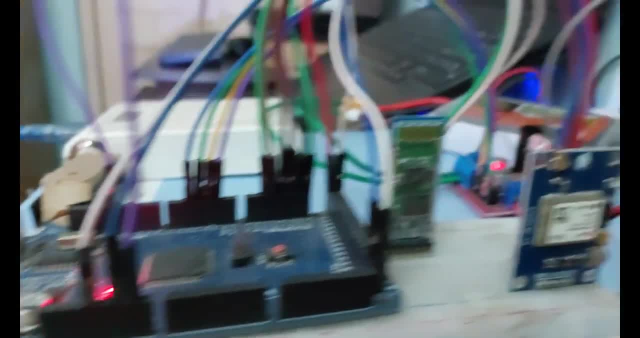 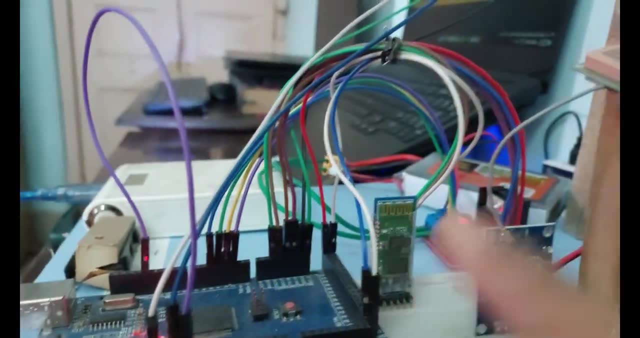 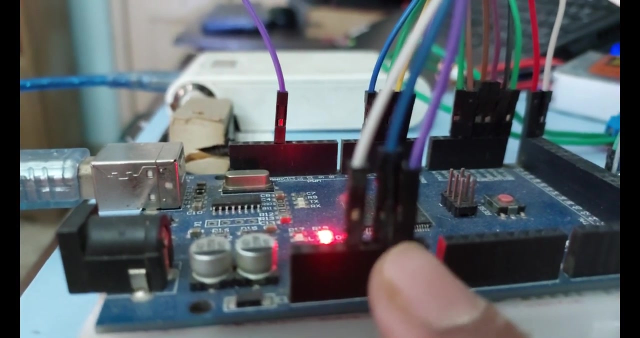 to the tx of the modules. basically, you have to reverse them. other than that, just power up the bluetooth and the gps using 5 volts and ensure to connect the compass up there down here into 3.3 volts. as you can see, this is the compass and this is the compass ground. this one here is obviously the ground for the main. 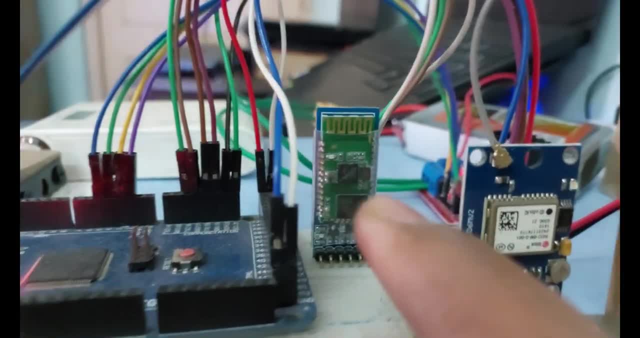 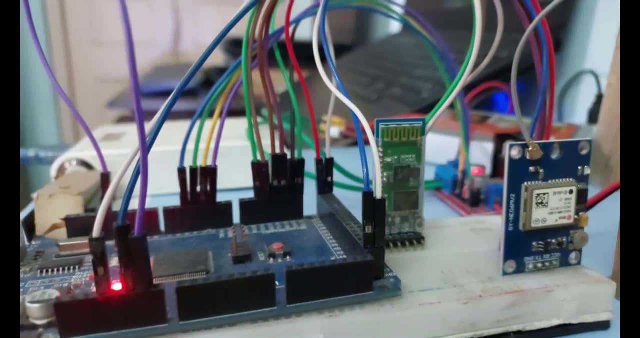 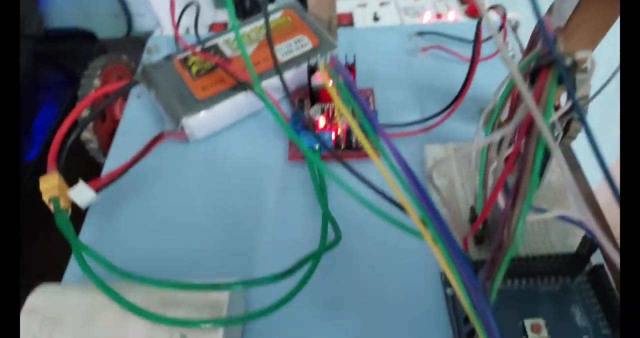 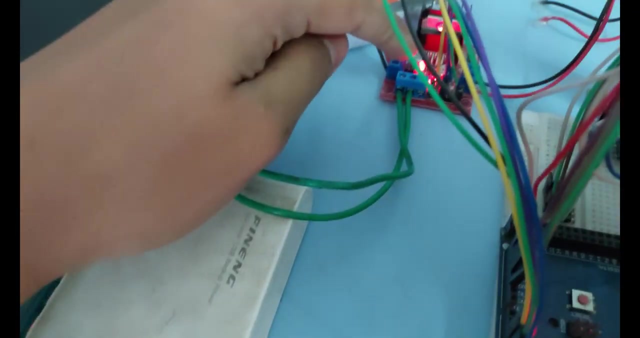 microcontroller turning on the motor controller, and then here we have the grounds and ground here and vcc back there for the gps, as well as the compass- i'm sorry- the bluetooth now for micro control for wiring up the motor drivers. basically, we are just using digital pins, two to five, as you can see there. so i'm not 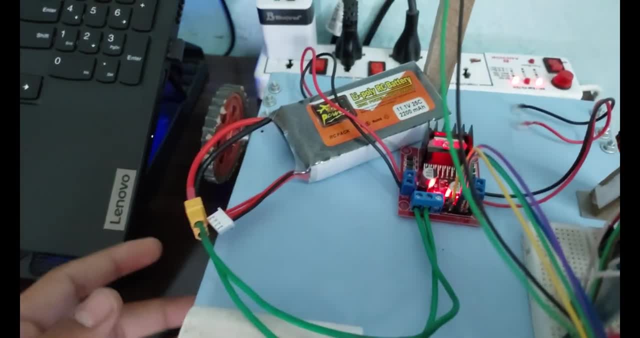 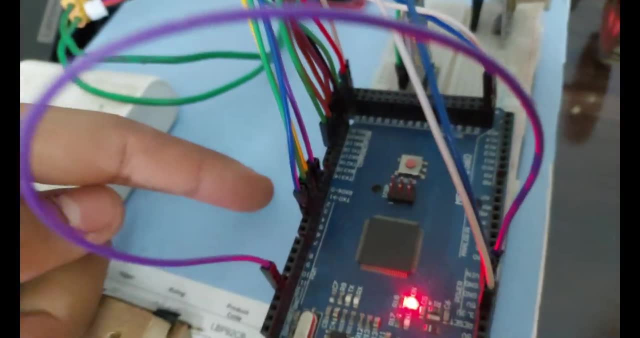 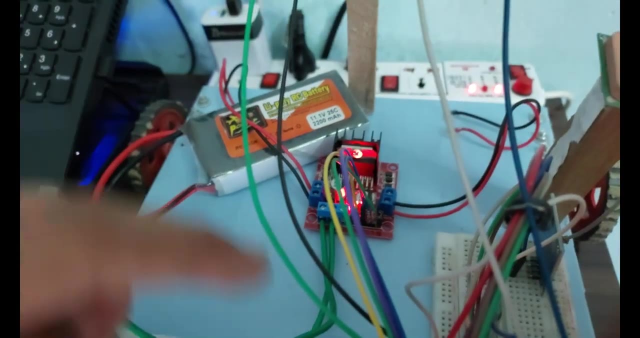 using pwm, as this is quite a heavy machine and the motors need a full- uh, full- power to run. however, the next two pins, which is five and six, are actually, in the code, set up as pwm pins, so you can just simply put your values in and connect those through there if you wish. so this on the 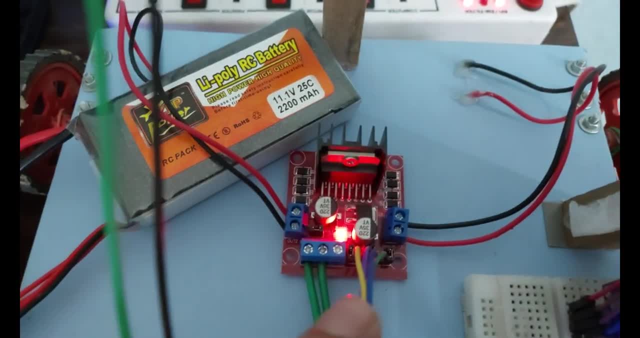 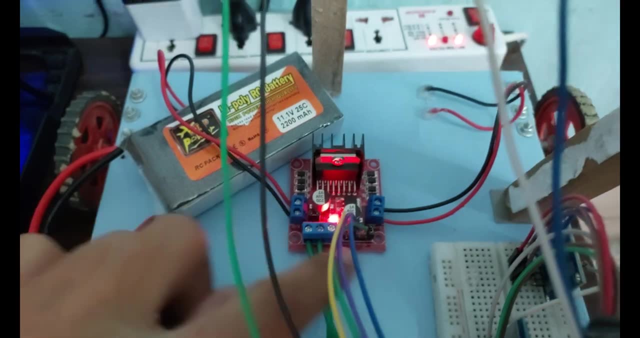 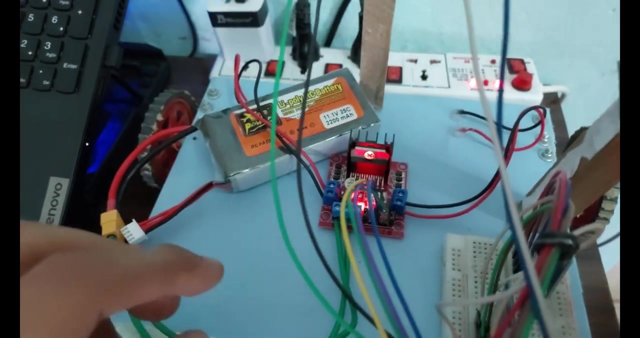 motor controller here. look, there is actually two jumpers. so you just remove the jumpers and connect up the wires on this side to pwm. this one is for this output and this side is for this output. just connect them up to the microcontroller on these two pins and you can have pwm output. now, if you are using a five, 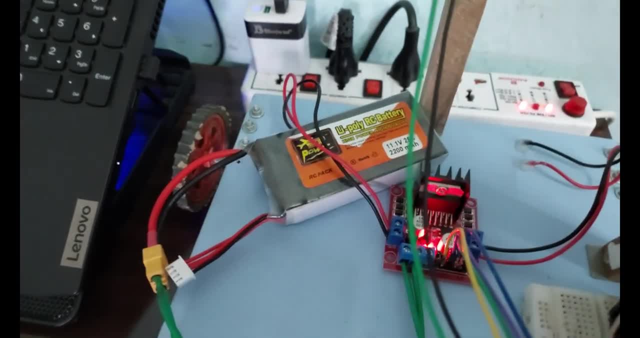 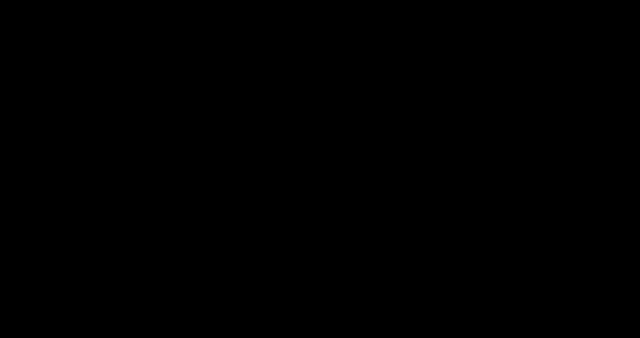 volt motor system and maybe a little lighter of a car you can get away with, directly powering this guy off of maybe another port on this power bank or something similar. however, i'm doing this other one basically powering off with this, because, uh, this is, i'm not really testing- in a very uh like. 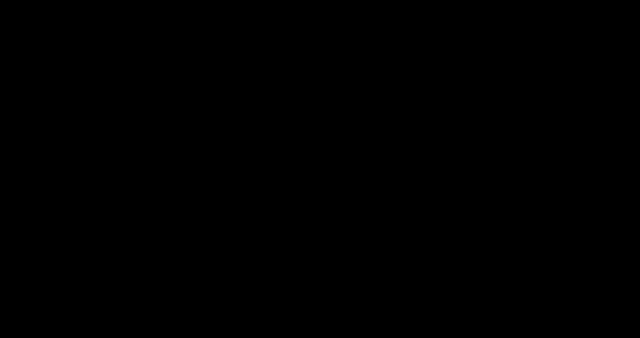 on a paved road. i'm actually going to a unpaved road. you'll see a little bit more about that later on. so that's why i need more higher power motors with, uh, more torque and stuff. so that's why i have to do this solution now. one more last thing about the gps is: be sure to keep this antenna. 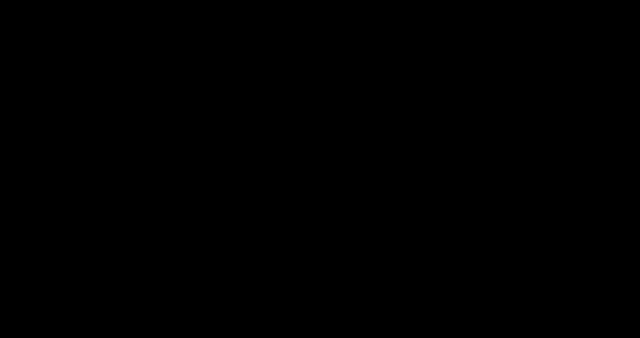 uh, this gps antenna a little bit higher elevated and also just make sure that it is clear of any obstacles above it, like don't cover it using anything. it actually needs direct view of the sky to properly work. this is a very low powered gps. it's quite finicky, so it doesn't work well. 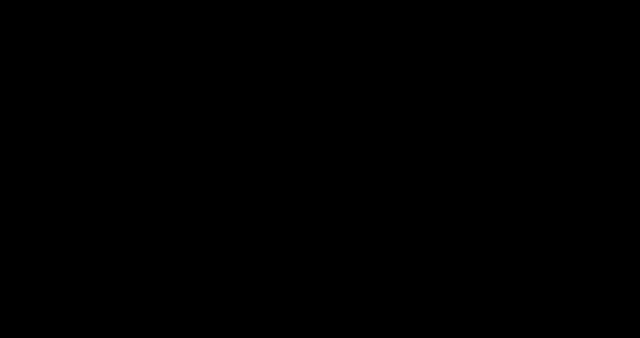 sometimes, especially if there is more like more obstacles above the gps antenna and stuff. so, as you can see, i actually have it a little bit angled on this piece of wood here, so it just helps it to basically just see this way instead of being covered by all of this. same goes with the uh compass. just use the a big pole and at least. 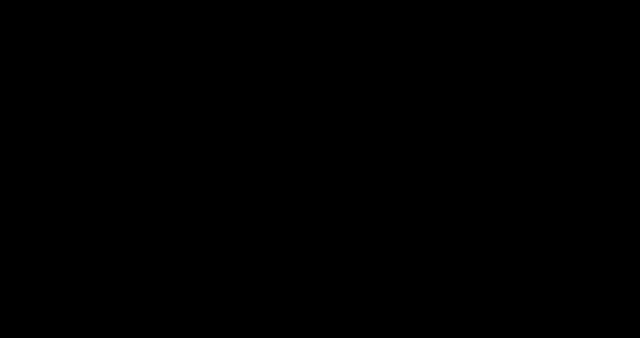 like separate it from any other kind of metal by at least 30 centimeters. this, i believe, is about 60 centimeters or 30, i can't remember exactly right now, but this is more than the required. so just make sure it's at least 30 centimeters elevated from the rest of the uh electronics. 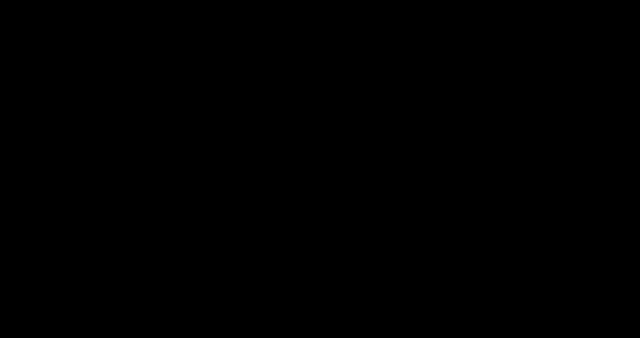 the reason is because these are all basically creating magnetic fields when current is running through the wires and this compass, the way it works, is by measuring of the magnetic field of the earth. obviously, that's how a compass works, so basically it can create interference on this compass, so that's why you want it to be as separated as possible from the rest of the things. 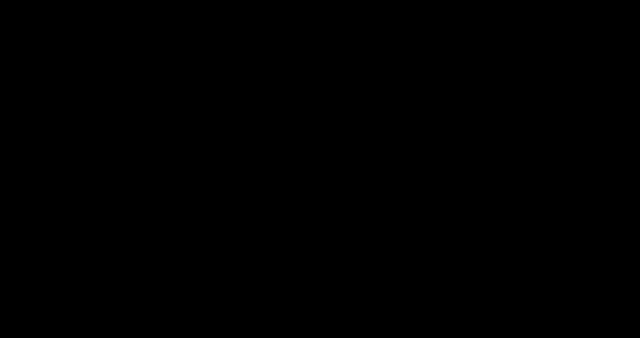 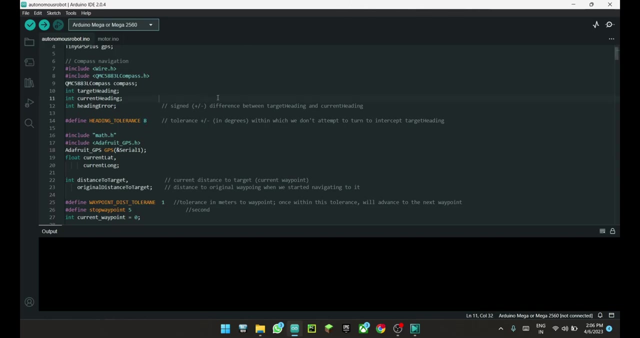 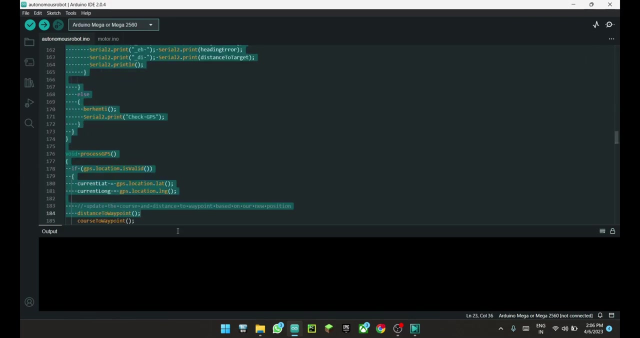 now, other than that, basically that's it, so i will quickly switch over to the code. i'll explain a little bit about the code and then i'll show you the video of this in the field. okay, so i have. now i'm quickly going to blush over this code, as it's going to be very long video. if i read all 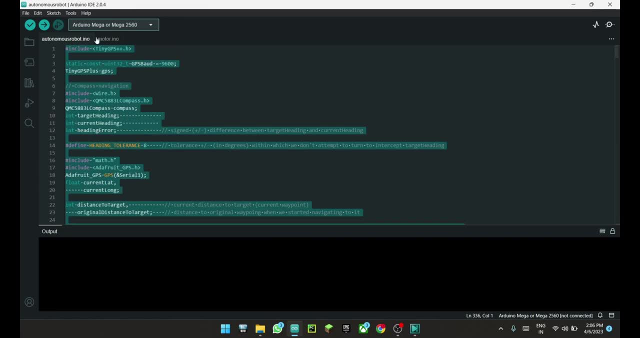 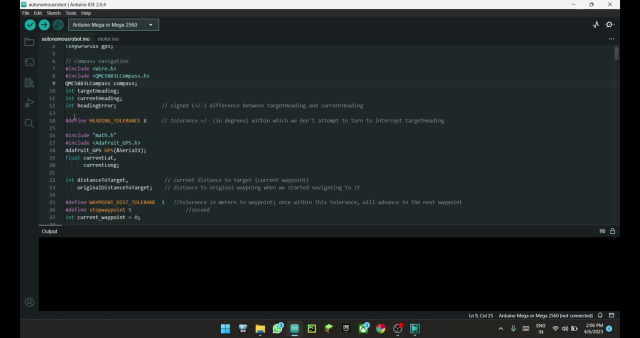 these explain all these lines of code, channel 35, as well as this part here. this is for your motor controllers. so first of all, let's just start off with the things you might want to know. so first is this one: this is your heading tolerance. this is, uh, basically how like in plus or minus eight. 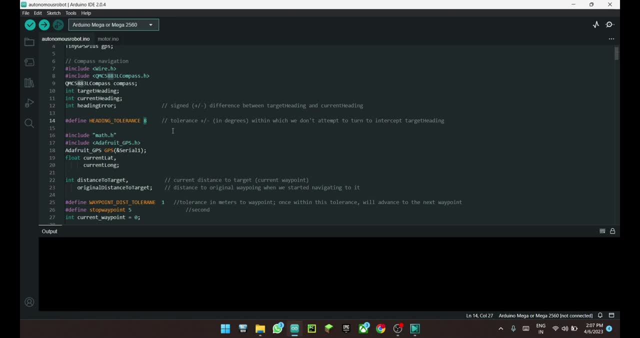 degrees. as long as your compass is reading plus or minus eight degrees from your target heading, it's not going to try and move it around. it's not going to move it around. it's not going to move it. the robot this. you can set this to a little bit lower if you have a little bit more accurate. 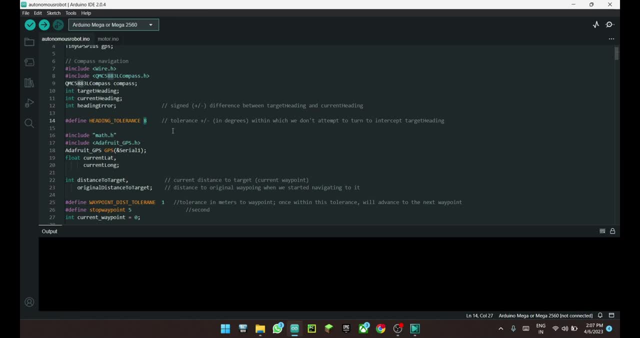 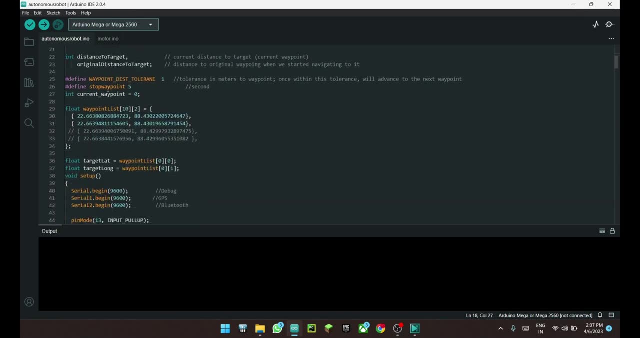 compass, or you can move your robot more accurately and a little bit higher if you have obviously the opposite. other than that, here we're just using libraries and initializing. this is one more thing you might want to know. this is a tolerance to your waypoint in meters, so as long as the robot 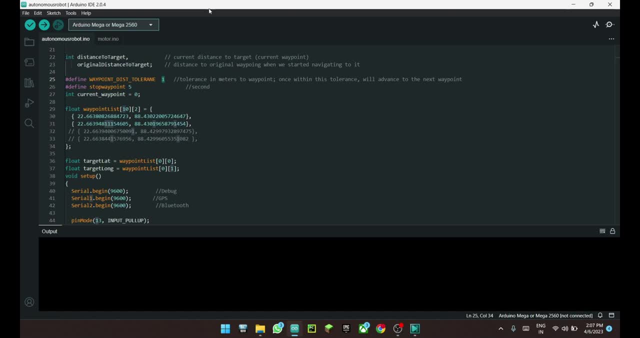 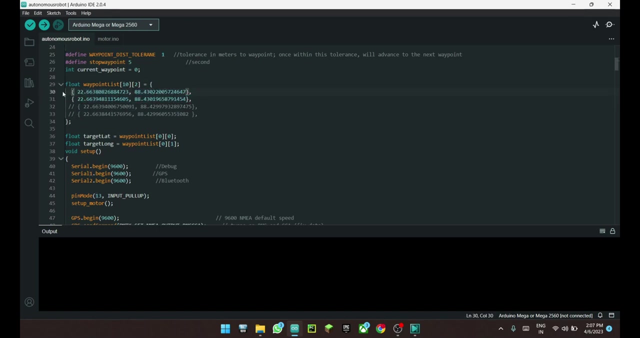 is within one meter of the um of the target. it will continue to the next waypoint, not trying to go any further down. you can again, based on your gps accuracy, you can adjust this as you wish. uh, here is your waypoint um. this is where you store all your coordinates. so the first one, this is the. 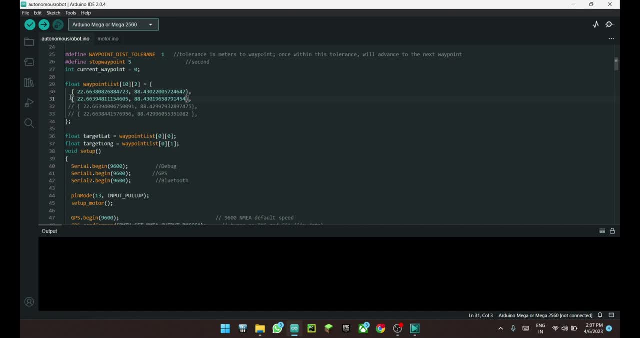 first coordinate. this is the second coordinate i had. i'm just using two coordinates for the test. even in the video, that is because of the condition of my ground. where i put the robot it was not possible to move too much. uh, the robot kept getting stuck. i'll show that a little bit more. 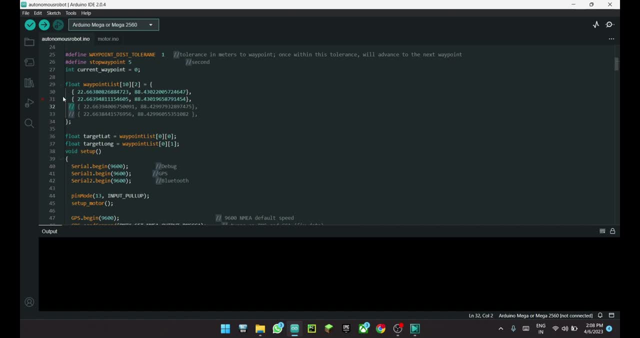 when i'm talking about the video of the robot moving. so i originally planned to do four. however, i ended up just doing two, one straight, turning around and coming back. uh, so this you can now have up to ten. in fact, you can have as many as you like, just change this number to whatever you want. so if you want to have, say, a, 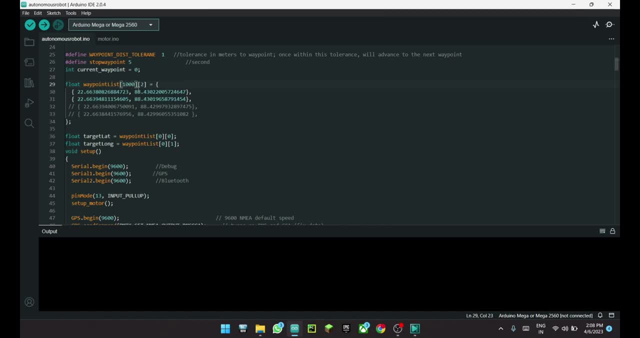 thousand uh waypoints. if you do, then you can change to one thousand. i have it ten, because i think no one realistically won't want it greater than ten waypoints. if you want more, just uh, just forward, just put this uh curly bracket and then put a comma and then continue up to ten and change. 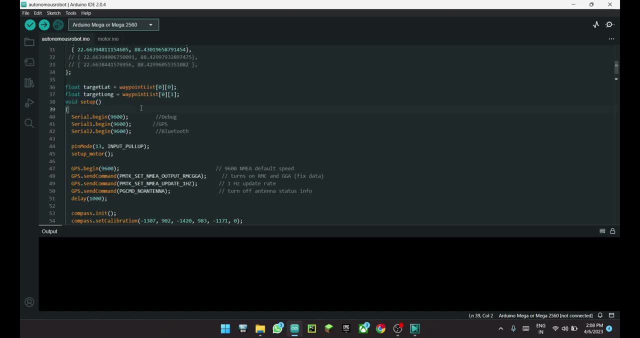 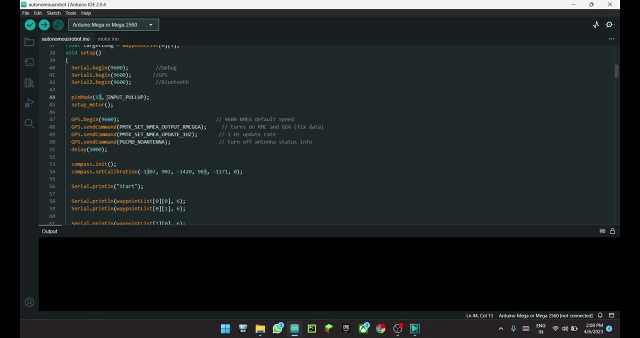 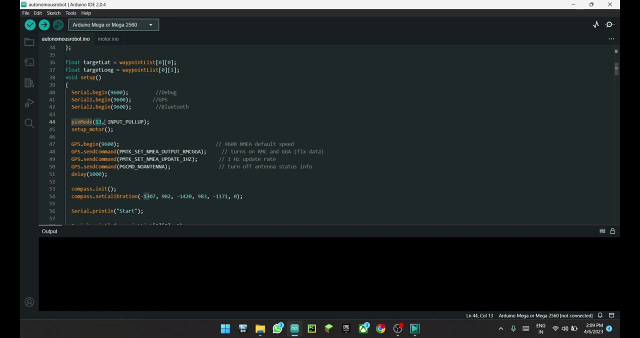 this. if you want more again, just more uh setting more float objects and then here cereal. this is one more thing you would like to know is: this: is your input pull up in? so i talked about this a little bit more when explaining the uh wiring of the system. so this is the pin which, basically, if 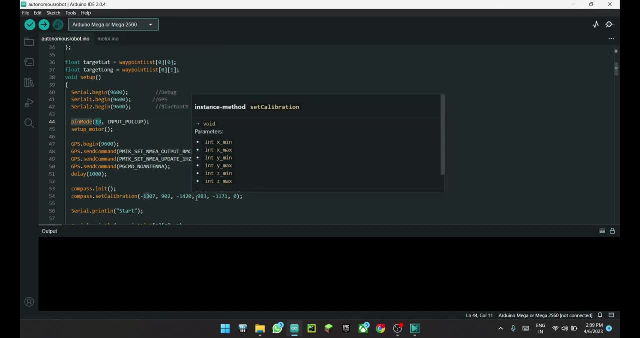 this is connected to ground. it will prevent the robot from moving. so you can set up the things such as the compass- uh sorry, not a compass pin. you can replace that with a compass pin. you just成 Course. there's no dever for simply focusing on the FlipS rumor. so you can place your robot. intro the 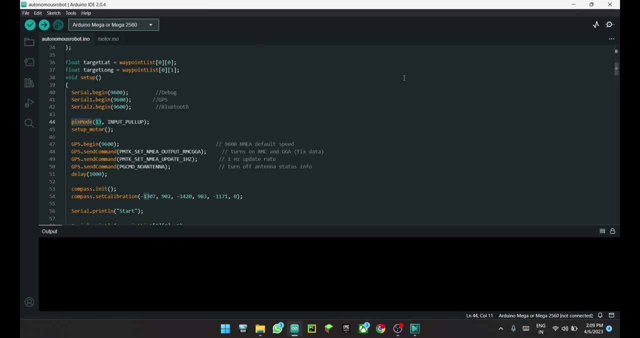 ło recipe option, as this is the one way so that we can pick up some. actually come over to the physician. we remember this is just the Curly Bracket, you can just use thisuwr shortcut. is then you difficult میALK criticism, a compass, the GPS, Bluetooth, etc. you can set up everything else, ensure that everything else is. 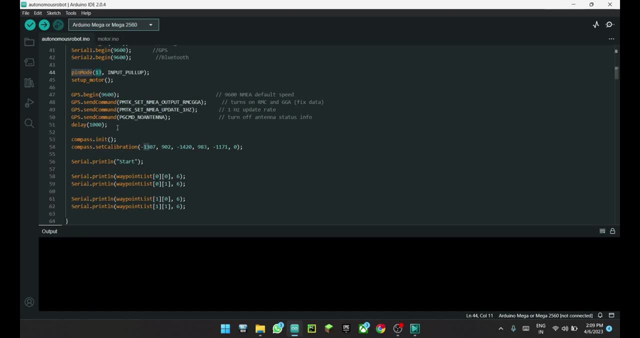 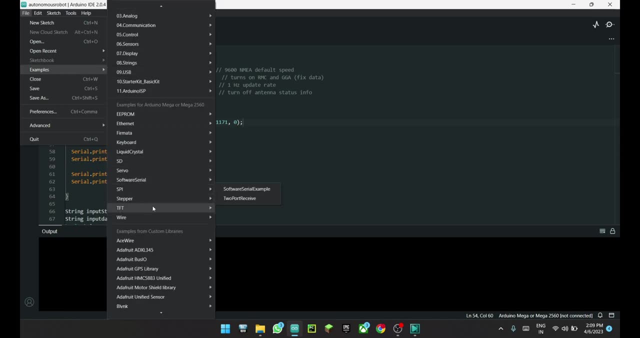 correct and then you can pull this so that what will start moving? uh, here you are going to set your calibration, so calibration is done using your own library. so, as i said, i'm using the qmc as uh the order done, hmc, it was delivered at qmc, but i'm using this qmc, private hl compass library. 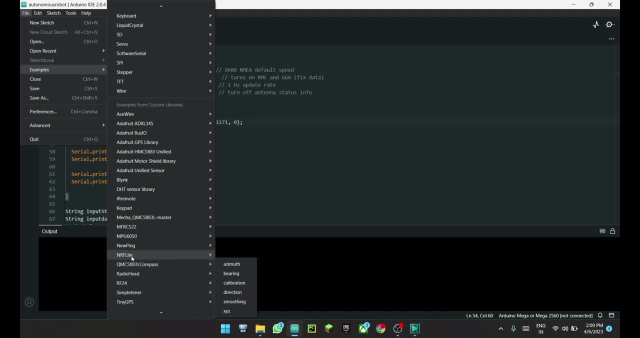 just search qmc private trail compass library and you'll get this one uh from github. now, here you're just going to use the calibration code here. just run that, move the robot around a little. just try and do it on its final position, as the amount of metal greatly affects the calibration. 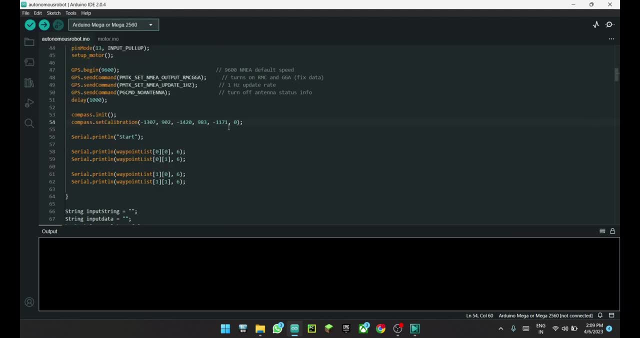 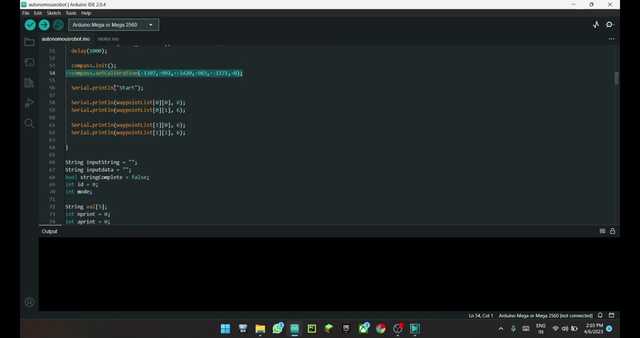 so just do that and copy the calibration and paste it here and the robot will be calibrated and your compass will be ready to go. then you can just here. we are just putting the way, sorry, just putting the waypoint list on to the serial of the computer for debugging, as well as just printing a start. 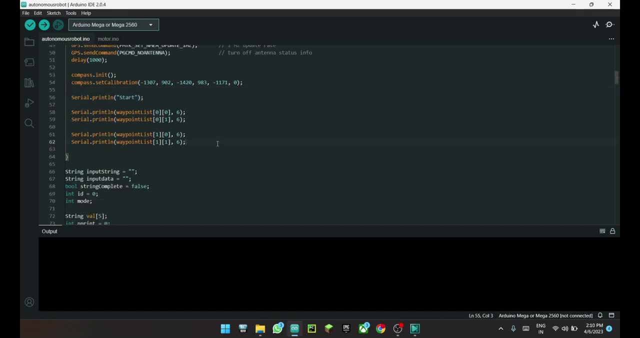 so you know it's going. uh, this is all for debugging purpose- is not really even going to be ever used, because obviously you're not going to have a computer connected to it. that's why we have the bluetooth and. but other than that, here we're just setting some more integers and 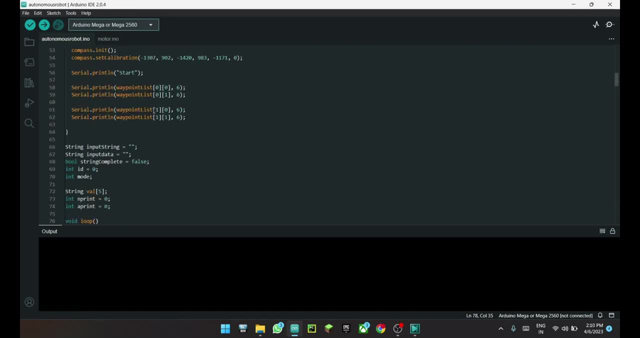 this is the part where we read the digital pin. so if you decide to change this for some reason from 13 to some other pin, make sure to change this one too, and the both of these you have to change. you know the dot of the pin. this is just the Registered Pin, so just. transfer for that part. so add only first part pin and then simply to see Peters, and here you can see, when you are just reading your serial, then you're just saying if serial is available, that is, if the GPS is read, then you have to read the serial and process the gps. then here we are, just doing more calculations and checking that everything is working. as you will expect. this is the part where we checked whether the part is connected to ground or no, time being 13. so if it is connected to ground, then obviously we don't want the robot to move and we'll just then count regular. whatever part. we are printing, some roundman speaking, we will now print some regular, a similar all. we'll just print in some regular old. 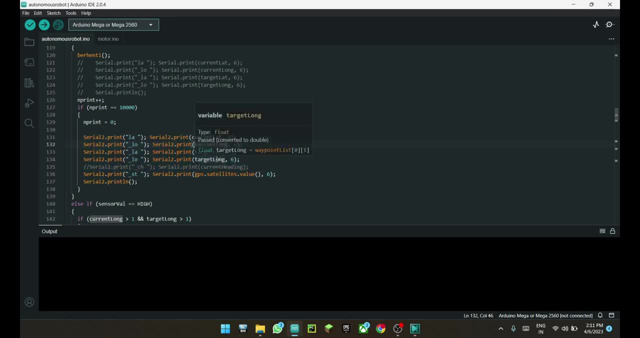 diagnostics. so current latitude, longitude, target latitude, longitude- this is commented out. this is printing your current heading. however, this will not work in this state. it will just freeze that last known current heading and if it is just you're starting fresh, then it will be zero. the reason is because the compass is being called later on in this other part when it is high. 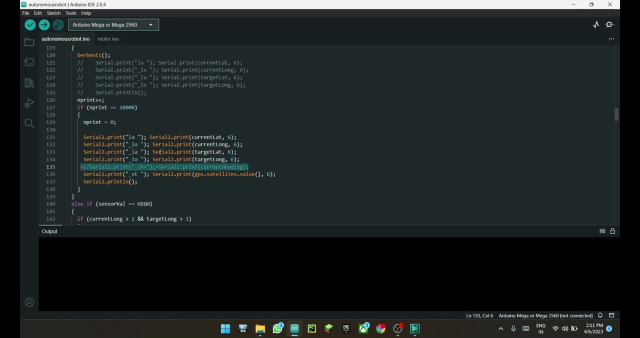 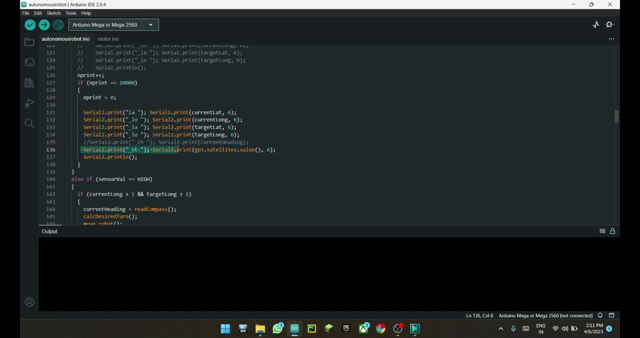 so here it just freezes the compass heading. it's the compass is not actually being called and it's not actually sending its headings to the robot at this point. and we are just setting the number of satellites in view and again, if it is high, that is, it is not connected to ground and assuming 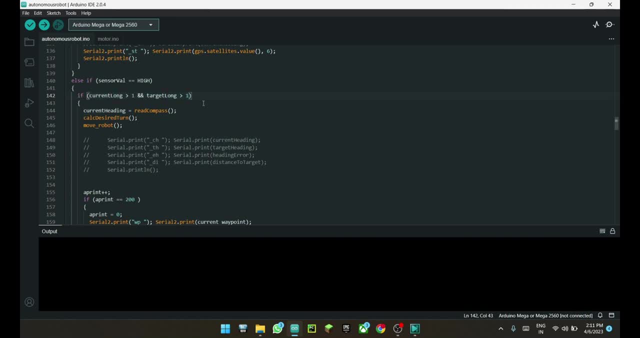 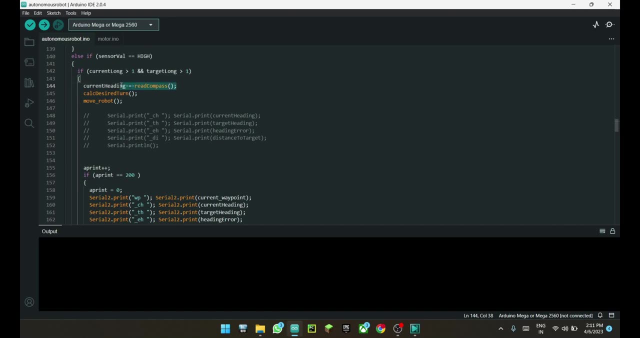 your current latitude and longitude is greater than one, that is, the gps is receiving satellite lock and it has uh, uh, it is getting your position. then we are going to read the compass, calculate the turn and move the robot and we are also going to print more uh diagnostics onto serial. so we are 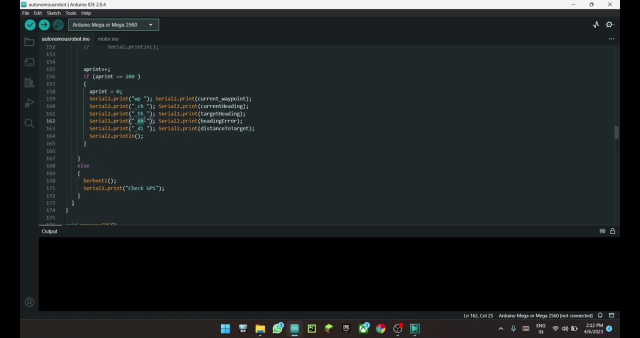 going to print the current waypoint: number heading, target heading, error heading. this is: this is basically your target heading minus current heading. that is, how much you are deviated from the target heading and your distance target, if it is not, however, greater than one. so this else is for this. 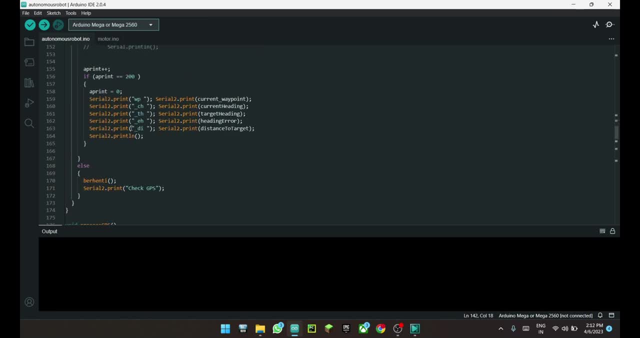 part current heading is greater than one, that is, if it is not greater than one, then it will be zero. zero, which means your compass, sorry, gps- has not received position lock. it will just print in a check gps, uh error onto the, onto your uh serial, uh, sorry, google. then here we are just processing. 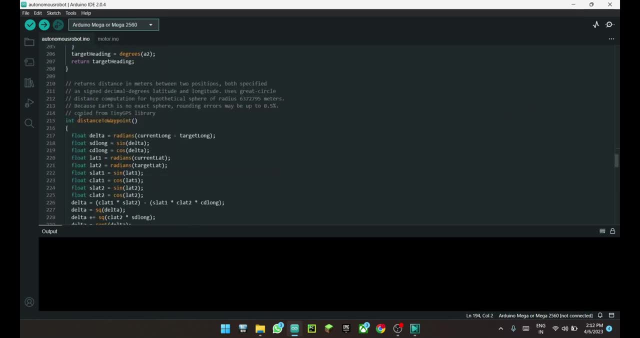 your gps calculating the course to waypoint, calculating the distance to waypoint and further. we are reading the compass here. this is one more part you might want to change if using a hmc. however, i'll leave the hmc link down in the description, the hmc code as well. so 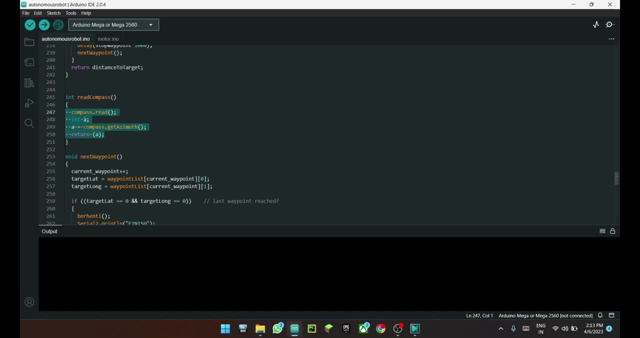 you don't really have to mess around with this, but this is one more part where you will have to change this from hmc library to hmc library, if you wish this. we are just calculating whether we are at the current waypoint or we need to progress further. if we are at the current waypoint, then we 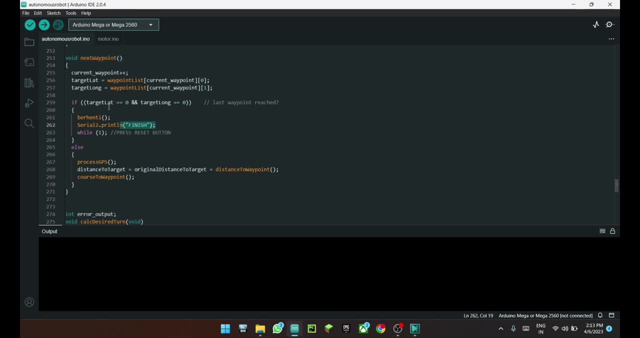 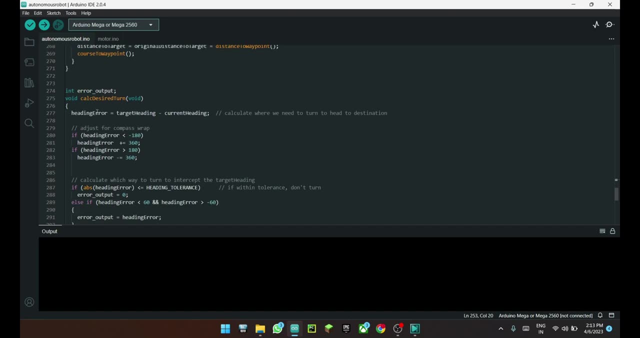 are going to finish. sorry, this is the last waypoint. we are going to put a finish on serial and wait for the reset button to be pressed. otherwise we are going to move to the next waypoint. we are calculating the desired term, that is, we are calculating our heading error. 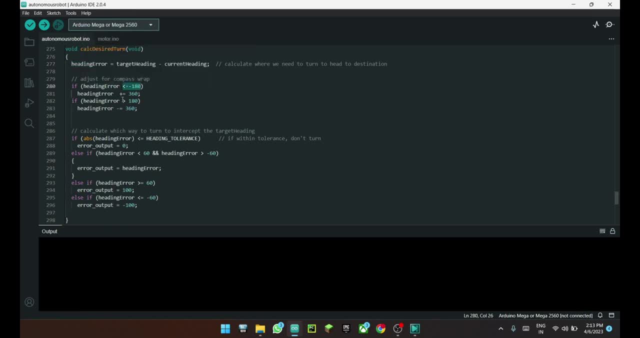 if heading error is less than minus 180 or greater than my 180 degrees. that is when, when it is greater than 180 means like you have to turn more than like. basically, what it's trying to say is: you have to turn more than- um, you know, you have to turn more than uh, like full circle, if it is greater than 180. so 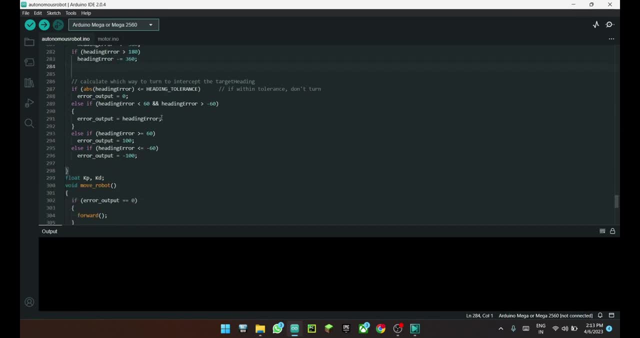 you are just going to have to set it to plus 360 or minus 360 respectively, to make sure it doesn't just keep spinning around, as that is what happens if you don't do this part. now, this, we are just setting some more limits to make our lives easier later on when moving. 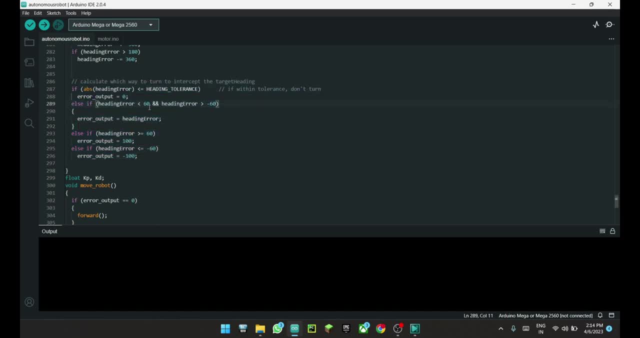 the robot. so if heading error is less than 60 and it is greater than minus 60, we are just going to set it to the error output to be equal to the heading error. so it will be between 60- sorry, it's 59- and the minus 59 here. that will be an error at this stage if it is greater than 60. 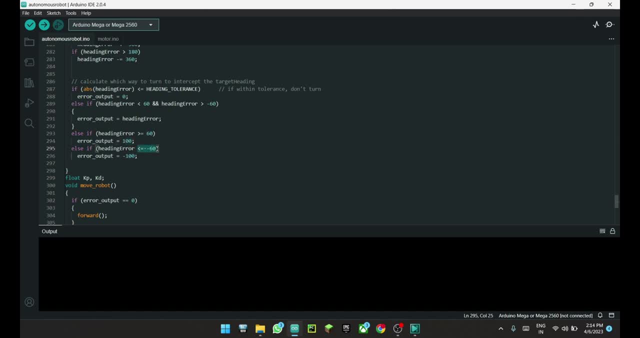 you are just going to set to one single value, 100, and if it is less than anything, less than minus 60, going to set it to minus 100.. this is going to be useful here in this part where it is we are moving the robot. remember we called for this up there in the code where we checked for the uh pin 13. 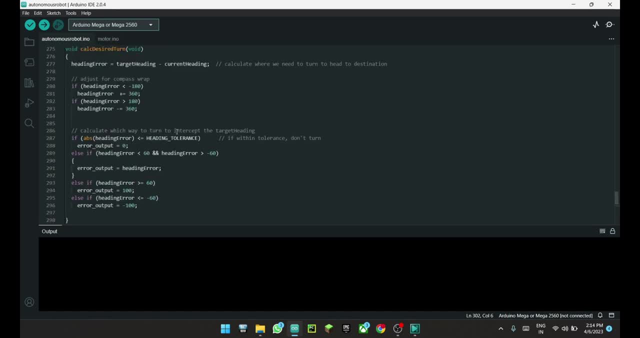 so, again, if it is equal to equal to 0, that is, if it is less than heading tolerance, your header heading error is less than your heading tolerance, which currently is 8, and it's just going to set your error out to be 0.. if it is the case, then you are going to move the robot forward. otherwise, if 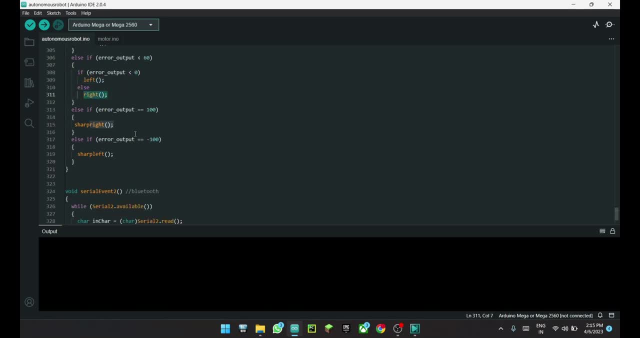 it is less than 0, you are going to move left, otherwise we are going to move right. if your error output is equal to 100, then we are going to move sharp right. that is now the difference, and if it is less than 100 minus 100, we're going to sharp left. the basic difference between left, right and 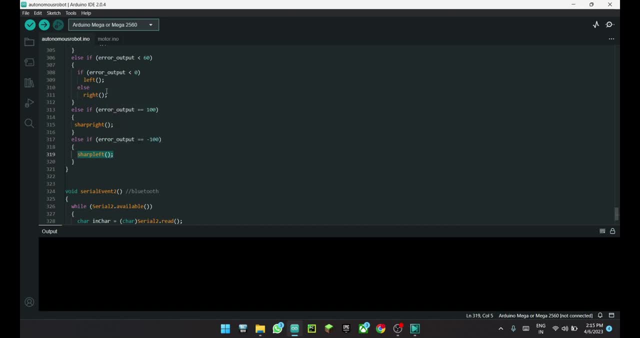 sharp right and sharp left is in left and right. we are going to move only one of the uh motors and basically it moves the robot more slowly if it is sharp left or sharp right. we're going to move two in opposite direction to make it move faster and come more. 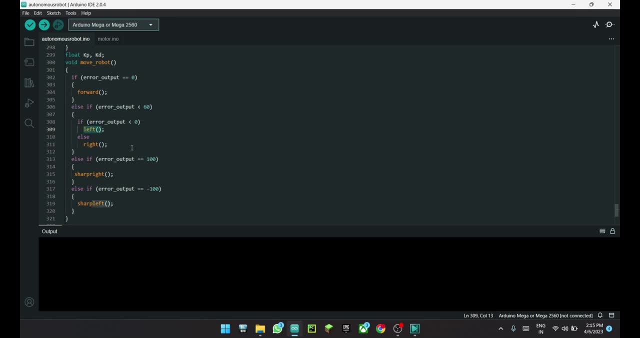 as long. as soon as it's less than 60, then we are going to just switch over to continuing only one model and get more accurate positioning here. this is just your bluetooth. we are just sending your bluetooth data and checking for bluetooth and sending the data as respective. this is your motor. 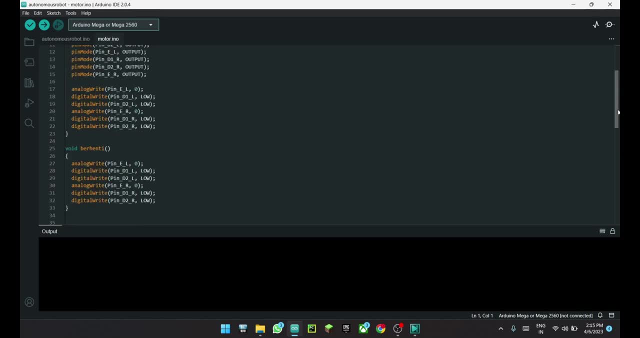 this other code. so this was the main code and this is the sub. well, like a sister code of sorts, you can say: this is where you are going to set all your pins for your motor controller, so these two are your enable pins, that is, pwm outputs. however, as i mentioned, 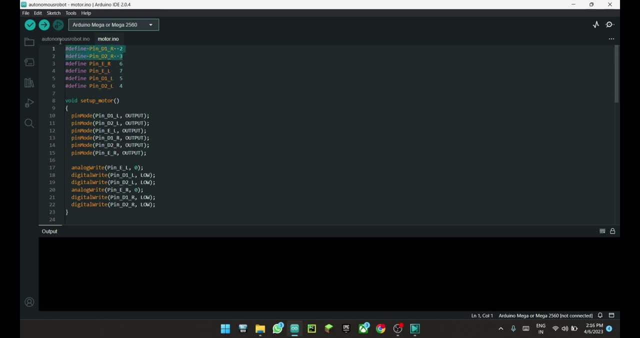 i am using full pdm, so these are not connected. and this is your left right motors and these are your left motor pins. you can mess around with this as you wish, based on where you plug it in. uh, plug the micro, the, uh, the motor controller into your mic. you are just setting all these. 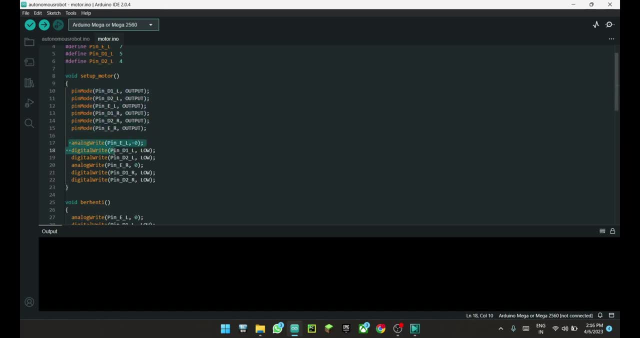 pins output here and by default we do not want the robot to move, so we are just going to set everything to low and the in the enable pins are going to be set to zero pwr. in baren hattie void was called uh here, if you remember, they were called at. if we are at the last viewpoint, then 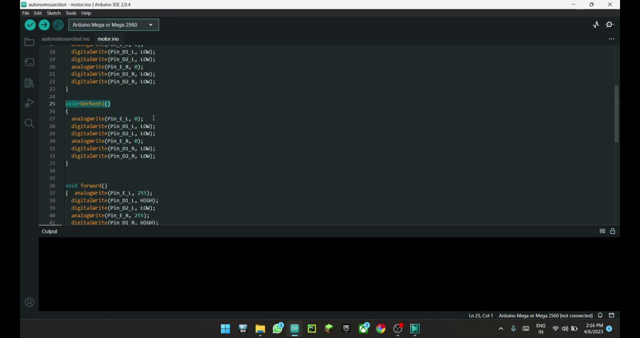 we are going to call it and other places up there, such as when the it is connected to ground in 13, this is just again same thing as here. we're just setting everything to zero and setting everything below to stop all motors from turning. now, uh, then we have wide forward, which is setting. 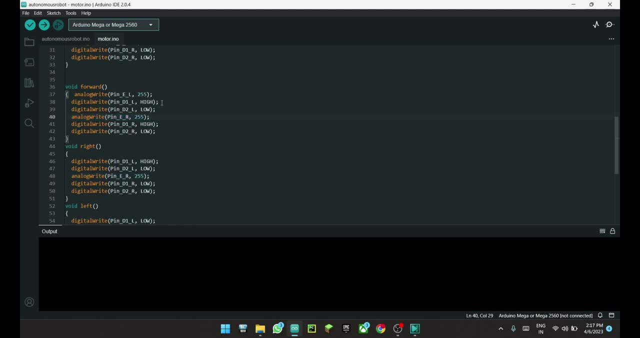 full power to both the and the enable pins and setting the for one of the left and right high set, moving both motors on the same direction. then, as i said, right moves only one motor and the second one stays off. then left you're again moving the other motor and